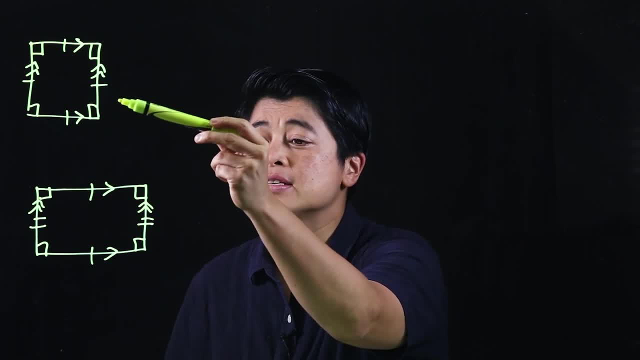 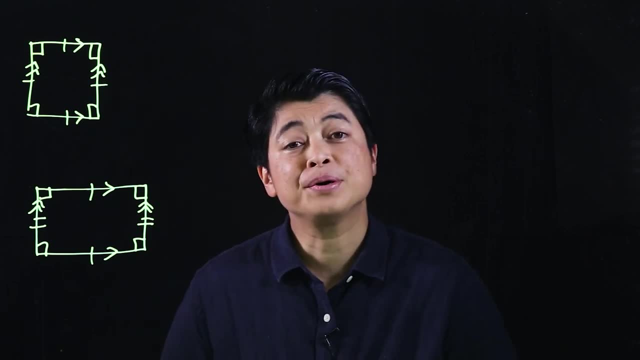 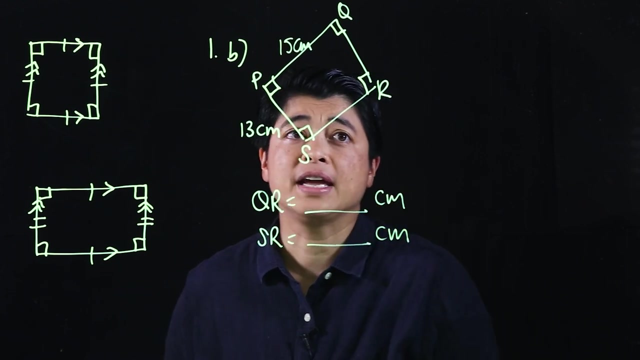 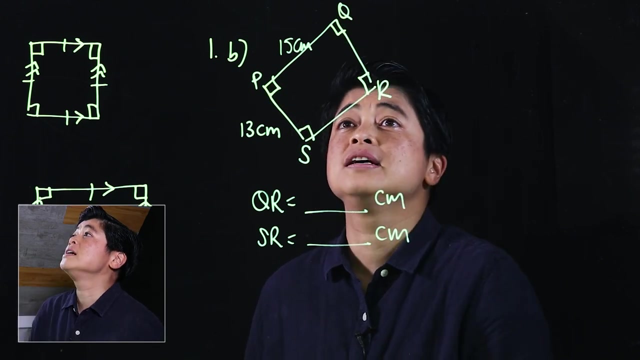 Which means all squares are rectangles but not all rectangles are square. Okay, so the exercises that we will be doing will come from two different pages. We start with page 102 and there's a drawing. Okay, Okay, So for this problem, it says that this side is 13 centimeters and this side is 15 centimeters. 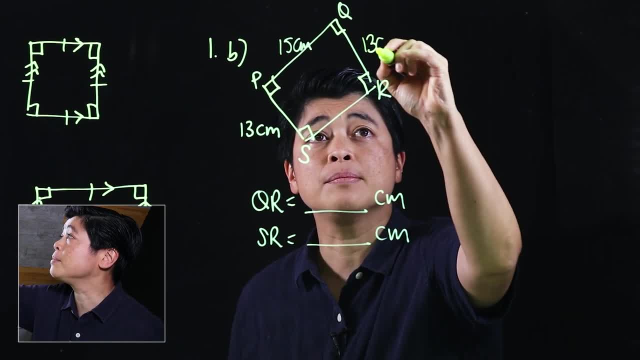 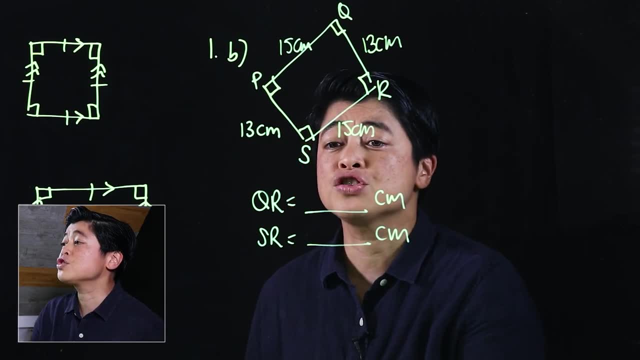 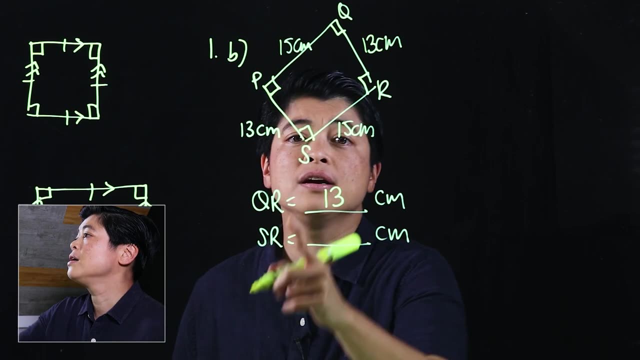 which makes the opposite side also 13 centimeters and the opposite side also 15 centimeters. So if the question says: what is the measurement of QR? QR technically is 13 centimeters and SR would be 15 centimeters. Okay, 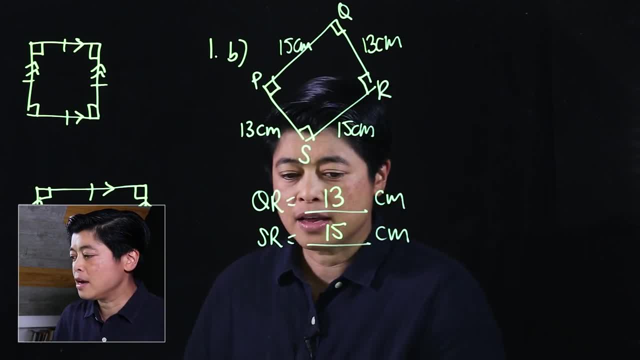 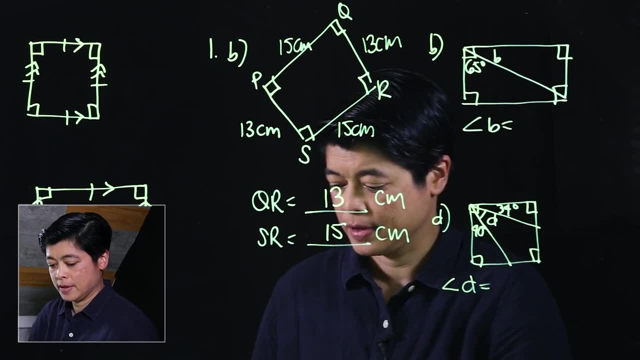 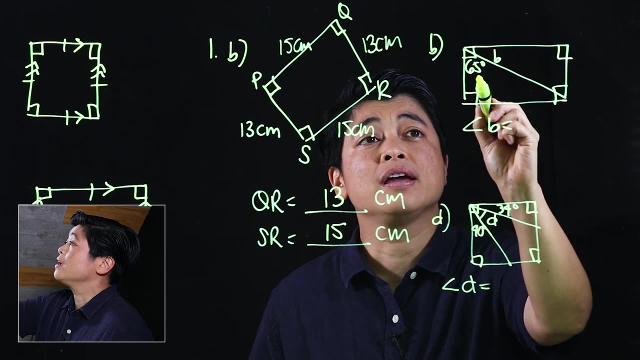 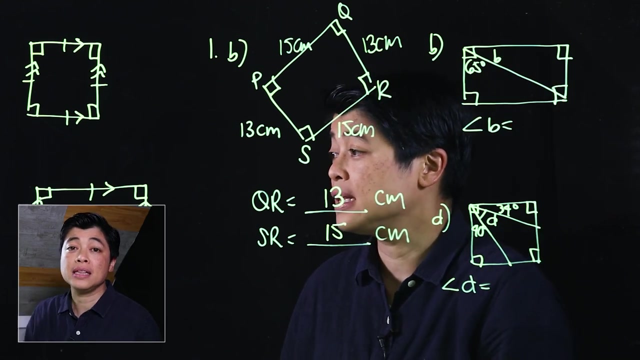 In page 104, again, there will be drawings. Okay, so let me draw them out. Okay, so we know that each of these angles are 90 degrees. So therefore, if it's divided into two different angles, then that means the total of the two should be 90 degrees. 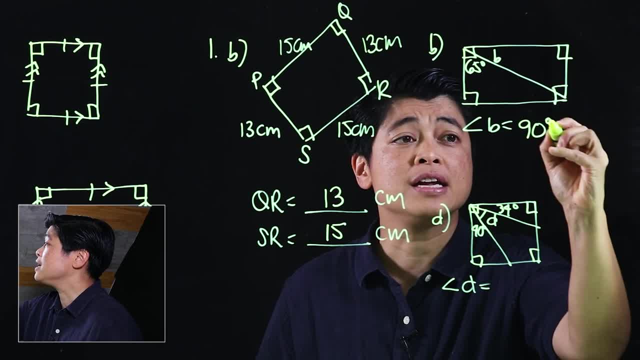 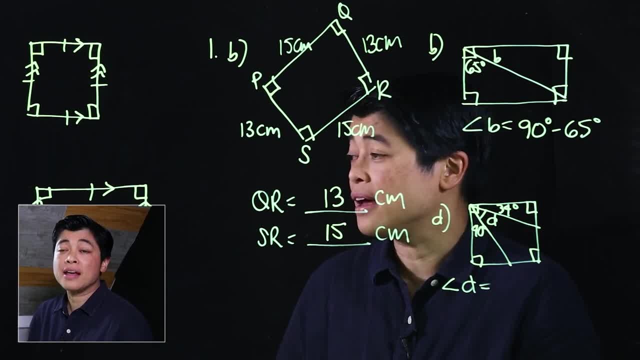 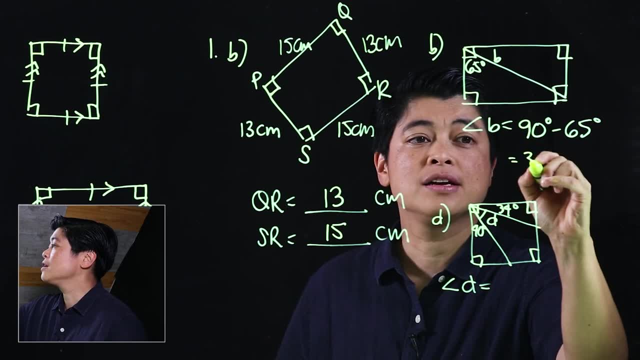 Now, if we remember our mental math, the way to go about this is: we subtract the tens: 90, minus 60 is 30. And then, since that's bigger, then we go like this: So this first, and then we go backwards. 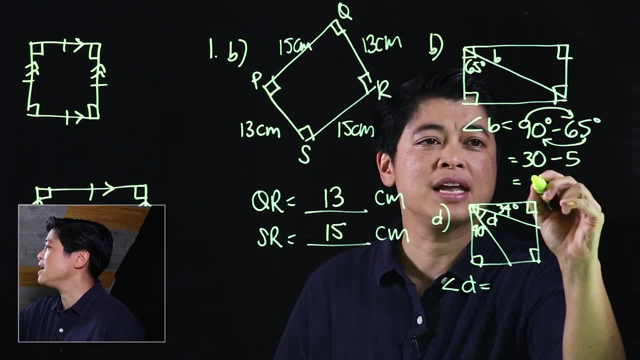 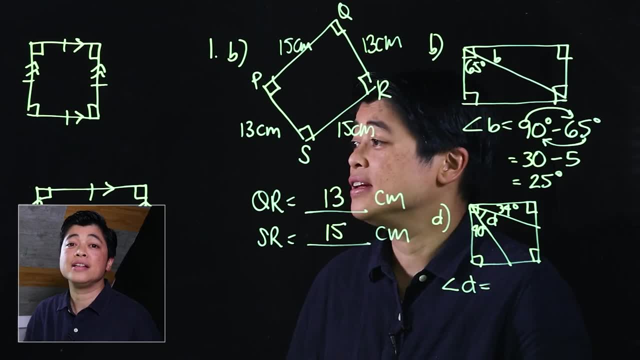 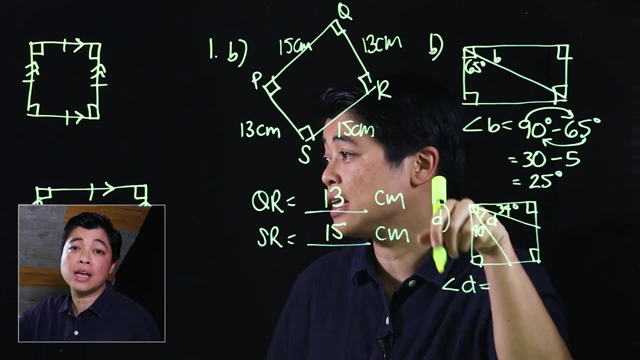 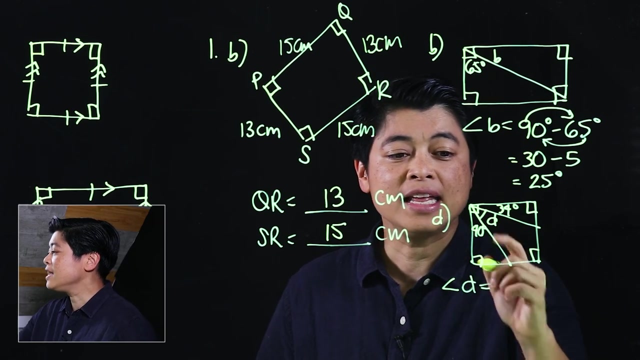 So this is minus 5, which means this must be 25 degrees. Okay, So making angle B 25 degrees. so if you don't know this strategy then you have to do it computationally. so write it down vertically, okay, in. let in letter d: angle d technically is 90 degrees minus the sum of